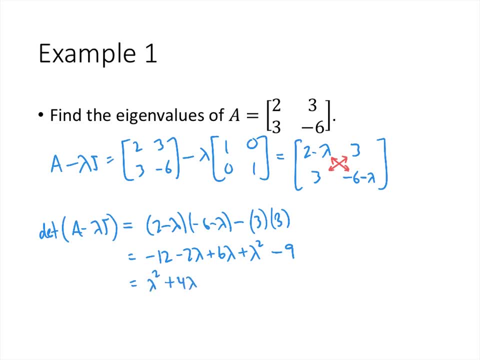 that's going to give us lambda squared plus 4 lambda minus 21.. When we set that equal to 0, that's quadratic. we can factor it. we get lambda plus 7 times lambda minus 3, that gives us two solutions: lambda equals negative 7. 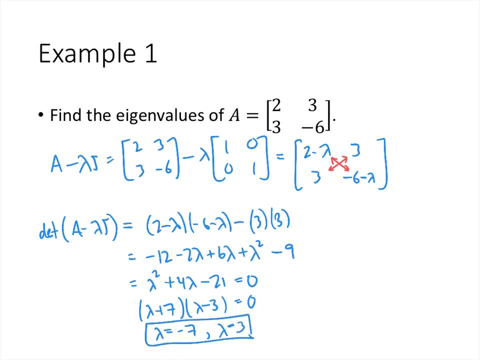 lambda equals 3.. So those are the eigenvalues of this matrix. Now, if what we wanted, in addition to this, was corresponding eigenvectors, we would solve the equation a minus 3i times x equals 0 and the equation a minus negative 7i times x equals 0. We would solve those in the normal way, the way. 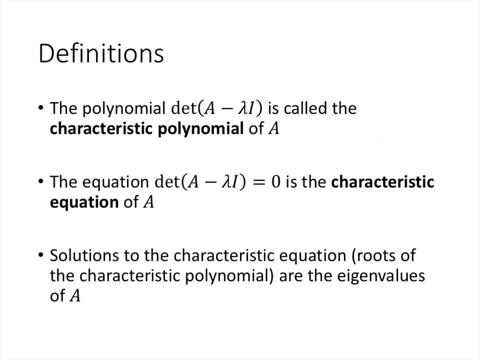 that we solve matrix equations, So a little bit of terminology here. So when we take the determinant of a minus lambda- i leaving lambda as a variable- what we get is called the characteristic polynomial of a. It's always going to be a polynomial and the degree of that 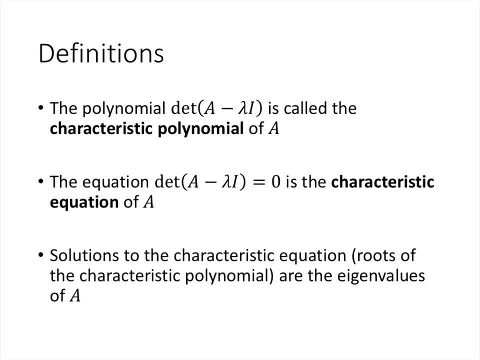 polynomial is always going to be the size of that square matrix a. When we set that characteristic polynomial equal to 0,, the equation that we get is called the characteristic equation of that matrix a And the solutions to that characteristic equation, which are really just the roots of the characteristic. 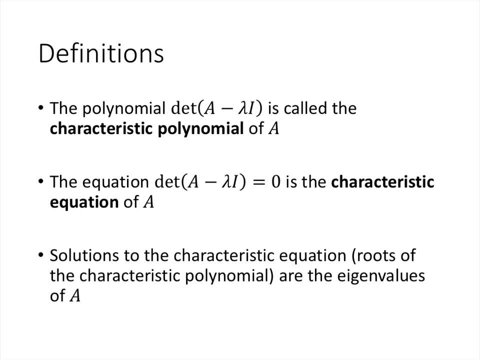 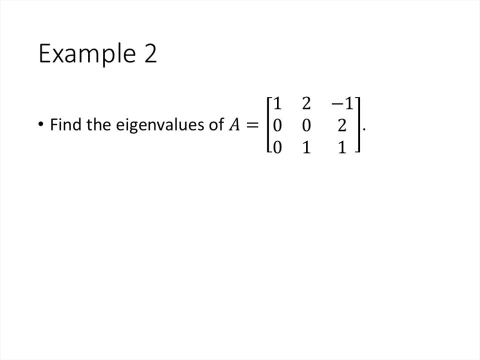 polynomial. those are the eigenvalues of the matrix a that we're looking for. Okay, let's do another example, this time with a 3 by 3 matrix. So now, when we take a minus lambda- i remember- all we're really doing is subtracting lambda from. 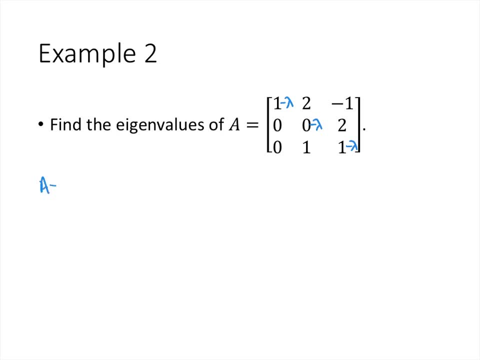 the diagonal entries. So that's going to give us the matrix 1 minus lambda, 2. negative 1, 0, negative lambda: 2, 0, 1, 1 minus lambda. Now we have to take the determinant of this three by three matrix as well. Anytime we have a factor who is 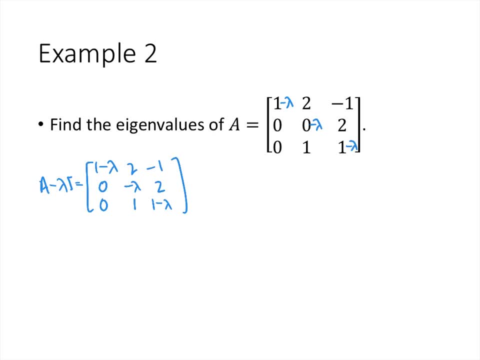 3 matrix and, as we learned a while back, that can be a little bit annoying, but what we're going to do is we're going to choose to go down the first column of this matrix because that column has a couple of zeros in it. So, using our 3 by 3 determinant technique, what we get is that the 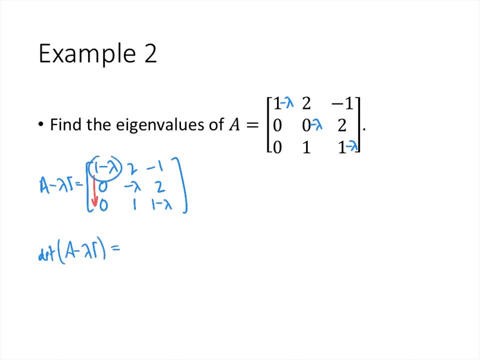 determinant of a minus lambda i is this entry: 1 minus lambda multiplied by the 2 by 2 determinant negative lambda: 2: 1. 1 minus lambda. That's going to give us 1 minus lambda. and then we're going to take that 2 by 2 determinant negative lambda times 1 minus lambda minus 2 times 1.. 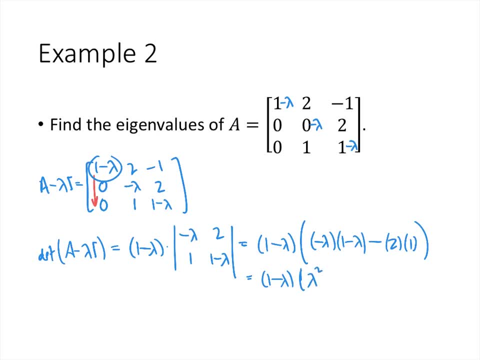 Inside those parentheses we get lambda squared minus lambda minus 2.. Now we could multiply this out, but remember, the goal here is to set this characteristic polynomial equal to 0 and solve, And the more we have that polynomial factored, the better. So in this case we have our 1 minus. 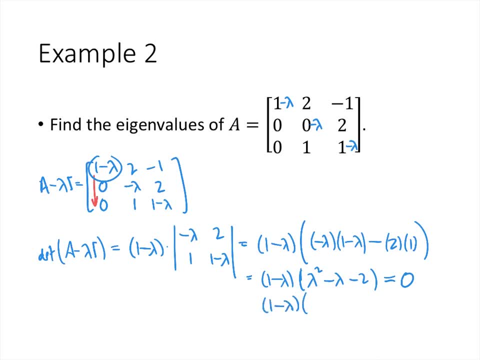 lambda factored out. we want to leave it factored out, and then we can factor lambda squared minus lambda minus 2 as lambda minus 2 times lambda plus 1. That gives us three eigenvalues: lambda equals 1, lambda equals 2 and lambda equals negative 1.. 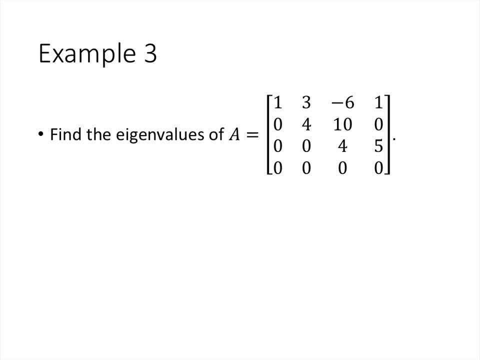 Let's do another example. This time we have a 4 by 4 matrix. but remember, a minus lambda i just means to subtract lambda from all of the diagonal entries. So a minus lambda i is this matrix: 1 minus lambda. 3 negative: 6 1 0. 4 minus lambda: 10 0 0 0. 4 minus lambda: 5 0 0 0. 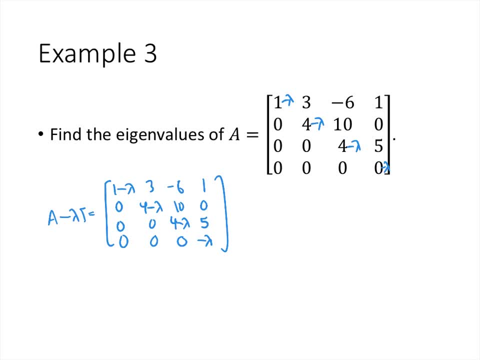 negative lambda. Now, taking a 4x4 determinant may seem intimidating at first, but good news here is: and finding the determinant of a triangular matrix, as we learned, is just as easy as taking the product of all of the diagonal entries of that triangular matrix. So in this case, 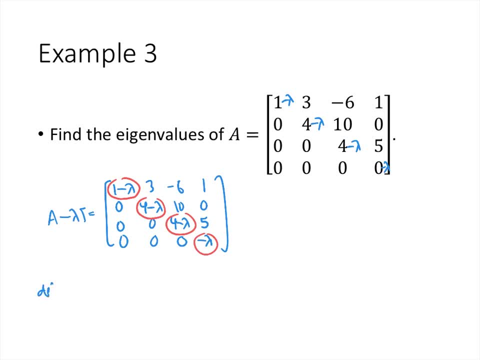 the determinant is actually pretty easy. The determinant of a minus lambda- i is just going to be the product- 1 minus lambda, 4 minus lambda, 4 minus lambda, negative lambda. And again we could multiply all that out, but that would be completely counterproductive. The goal here 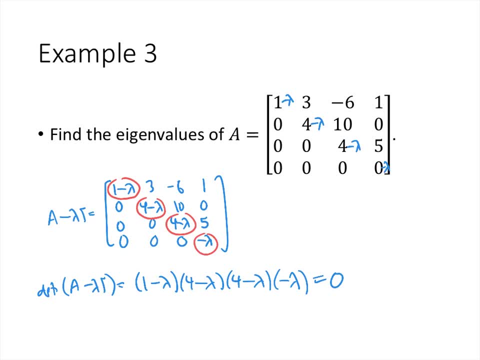 is to set this polynomial equal to 0 and solve, And so this, being in factored form, is exactly what we want. So what we get is: lambda equals 1, lambda equals 4, lambda equals 4, lambda equals 0. 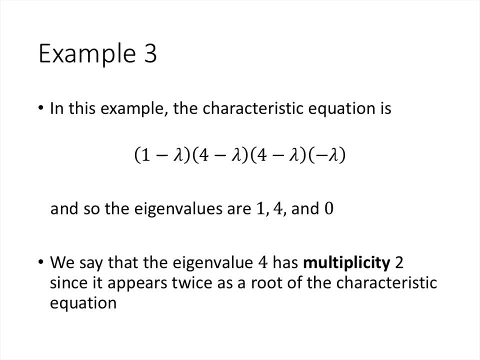 Now notice here that we get the eigenvalue 4 twice. The factor 4 minus lambda appears twice in the factored form of our characteristic equation. So we say here that the eigenvalue 4 has multiplicity 2. Because it shows up twice as a root of that characteristic polynomial. In this case we 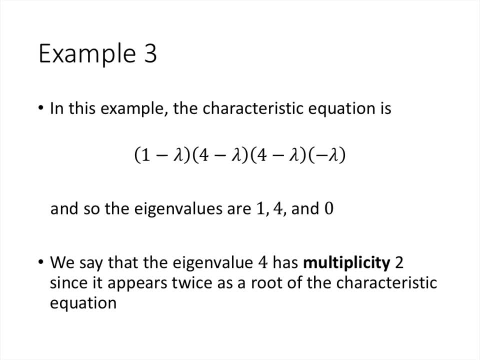 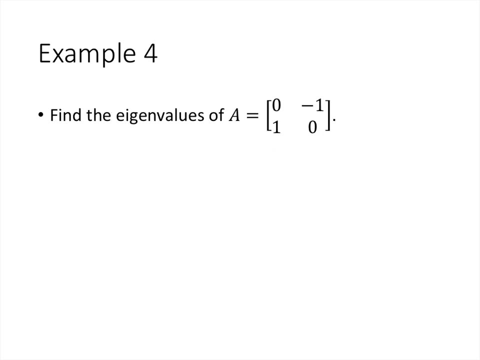 expect our 4 by 4 matrix to have 4 eigenvalues, because our characteristic polynomial has degree 4, and so we expect that polynomial to have 4 roots. And in a sense, this polynomial does have 4 roots, but only if we count the root 4 twice. Let's go back to a smaller example. 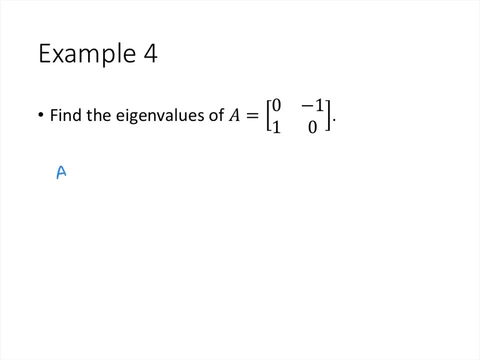 and see something else that can happen sometimes. So in this case, a minus lambda i is the matrix negative lambda, negative 1, 1 lambda, And when we take the determinant of a minus lambda i, what we get is lambda squared plus 1.. Now, when we set this characteristic, 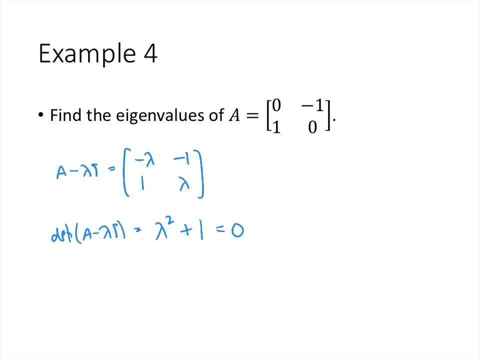 polynomial equal to 0,. there are two ways to think about what happens. One way is to say that there are no solutions. It's not possible to square a number, add 1, and get 0. But really what we mean when we say no solutions is we mean that there are no solutions. 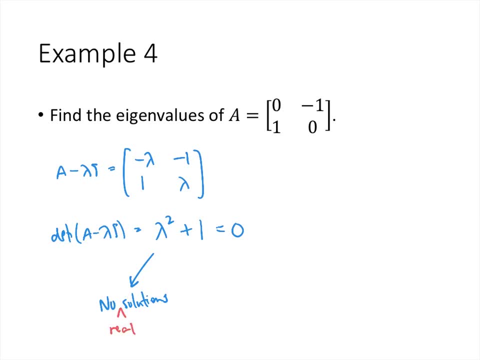 It's not possible to square a number, add 1, and get 0. But really, what we mean when we say no solutions is we mean that there are no solutions. So we can use the matrix to mean that there are no real solutions. There are solutions, they're just complex. 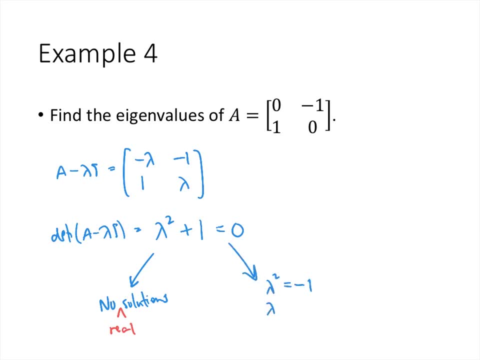 numbers. If we subtract 1 from both sides and take the square root of both sides, what we get is that lambda is plus or minus i, where i is the square root of negative 1.. So there are complex solutions, and so the question then becomes: do we allow complex? 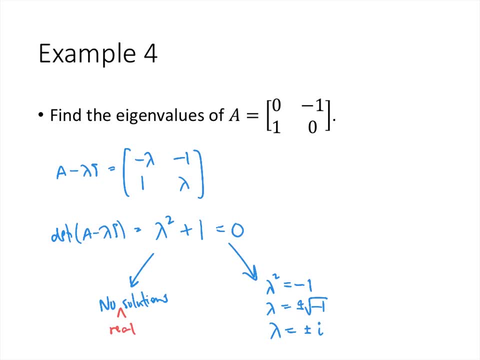 numbers to be eigenvalues or not. For the moment, in this course we're not going to allow complex eigenvalues, But we could. We could broaden our horizons, and we could broaden our horizons and open ourselves up to the possibility of complex eigenvalues. 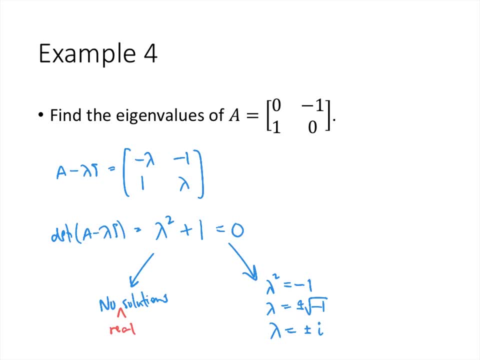 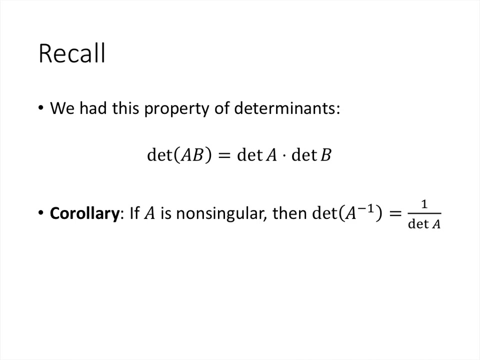 and then think about what the consequences of that decision would be, And that would take us down a whole other rabbit trail. but it's something to think about. But again, for our purposes we're not going to allow complex eigenvalues All right. now we want to talk about some general facts about these eigenvalues. One: 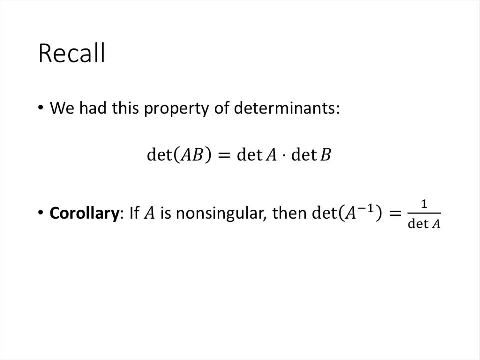 thing that we know from our discussion about determinants is that the determinant of the product of two matrices is the product of the determinants, And one consequence of that is that if you have an invertible matrix, then the determinant of the inverse is the reciprocal of the determinant. So let's think about why. that is Well the 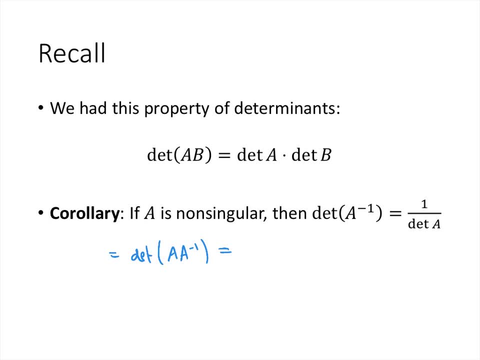 determinant of A times A inverse. there's two ways to think about that, Because the determinant of a product is the product of the determinants. that's the determinant of A times the determinant of A inverse, But it's also the determinant of the identity. 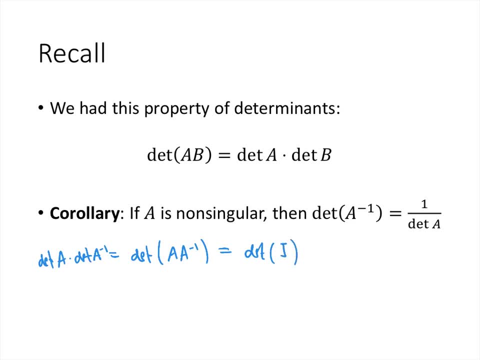 matrix, because A times A inverse is the identity matrix And the identity matrix as a determinant of one. So if I divide both sides by the determinant of A, I get exactly what we said in the claim that the determinant of A inverse is in fact one over the determinant. 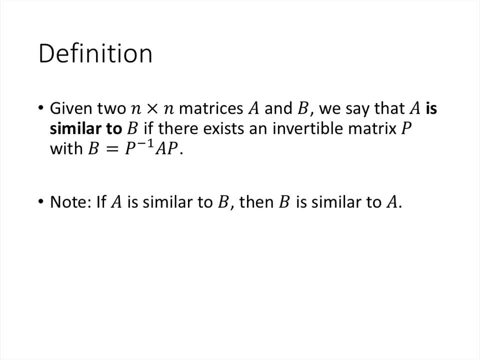 of A. Now we see that two square matrices, A and B, of the same size, are similar, That A is similar to B if there exists an invertible matrix, P, such that B equals P inverse AP. Now, for the moment, not sure what we're going to do with. 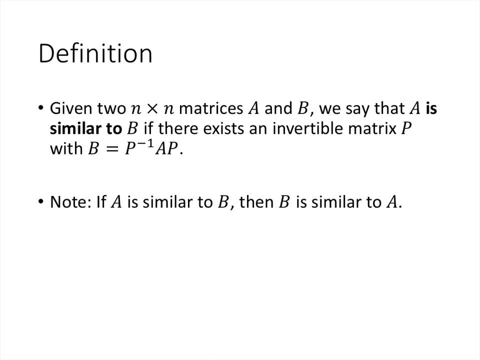 this definition but just try to understand the definition itself, and then we're going to use this a lot for the rest of this lecture and then in the next lecture. So is there a matrix, an invertible matrix, so that when I take A and multiply it on the left by P inverse and on the 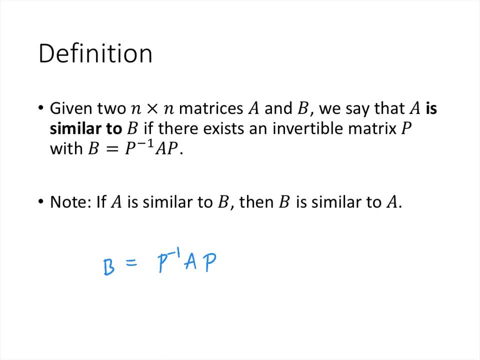 right by P, what I get is a matrix B. Notice that the P and the P inverse generally won't cancel each other out because matrix multiplication is not commutative. I can't swap the places of the A and the P to cancel out the P inverse and the P because I can't change the order typically with. 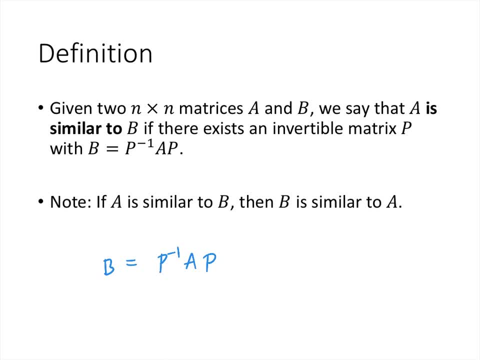 matrix multiplication. So we're not saying that A and B are going to be equal here. we're just saying that they're going to be in some sense similar, and we're going to get into what that means. But first of all, notice that if A is similar to B, then we can do the same thing. 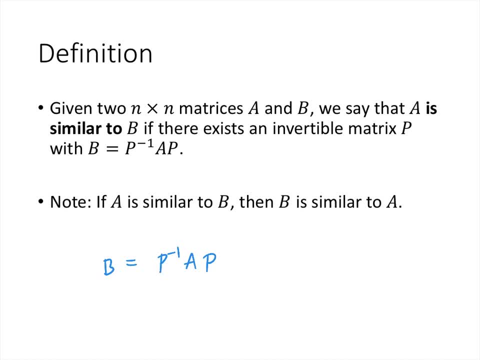 switching the roles of B and A, Because if I take the equation and multiply it on the left by P, and I multiply both sides by P on the left and P inverse on the right, what I get is P, B, P inverse, And notice that this P and P inverse since they're next to each other. that's just. 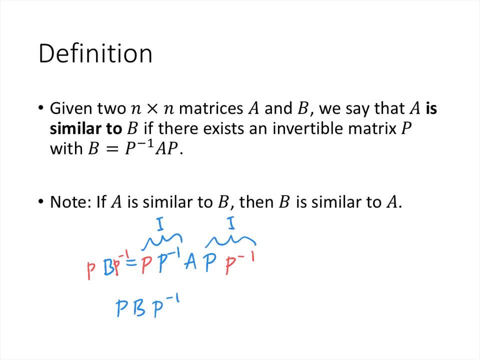 the identity, This P and P inverse, since they're next to each other. that's the identity, And so we get A. So this would tell me that A equals P, B, P inverse. Now that doesn't immediately tell me that B is similar to A, because I would have to have the inverse of a matrix on the left. 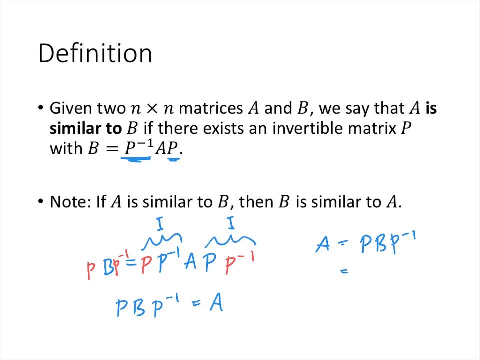 and the matrix itself on the right. But we can just let Q be P inverse, Then P is Q inverse and P inverse is Q. So this would show that B is similar to A. So if A is similar to B, then the similarity matrix, the P. we can just invert that and use that matrix to show that B. 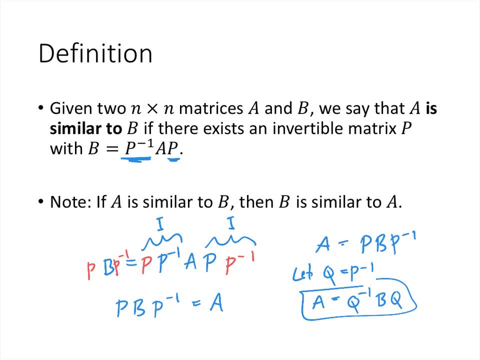 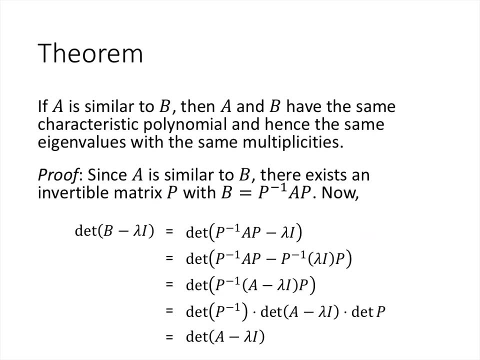 is similar to A, So we'll often just say that A and B are similar to each other, but without this little proof that we did here, that wouldn't have been quite precise. This theorem shows us something that we can do with similar matrices. 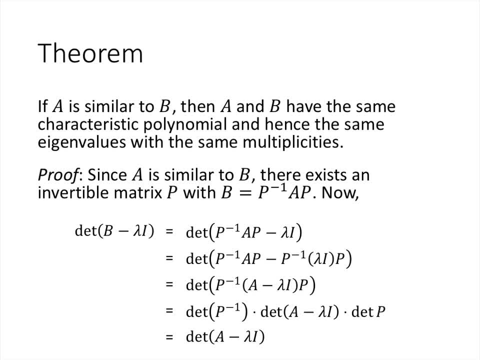 which is to note that if A and B are similar matrices, then these two matrices have the exact same characteristic polynomial, and that means that they would have to have the same eigenvalues with the same multiplicities, And so all we have to do is show that the characteristic polynomials are the same. 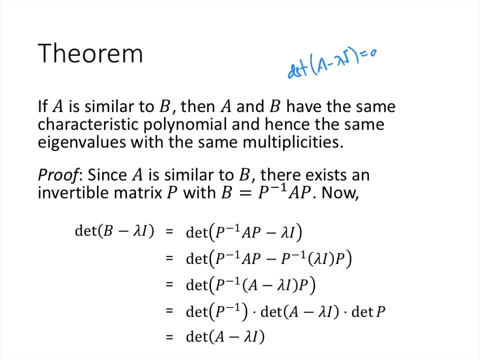 in other words, we have to show that the determinant of A minus lambda I is equal to the determinant of B minus lambda I. So we know that since A is similar to B, that B equals P inverse AP for some invertible matrix, P. 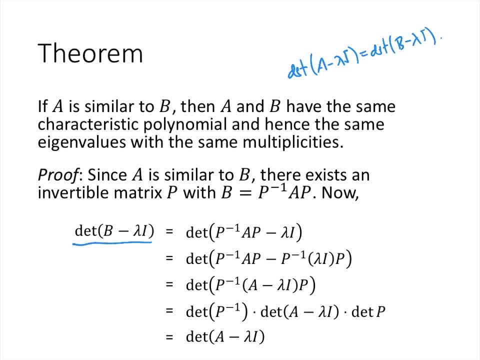 so we set this up. We've got the determinant of B minus lambda I. We're going to replace B by what it equals, which is P inverse AP. Now the identity matrix, and any multiple of the identity matrix commutes with any other matrix. 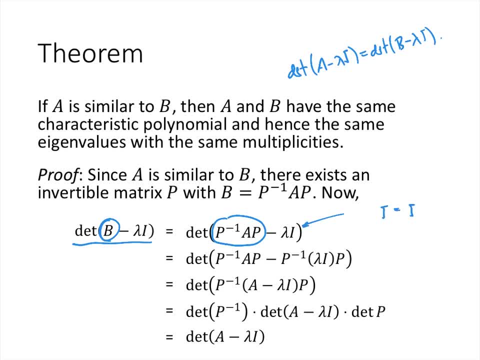 So here we're going to write: I as I times P times P inverse, because multiplying by P and by P inverse doesn't do anything. And then we're going to switch up the order, And then we're just going to multiply by lambda. 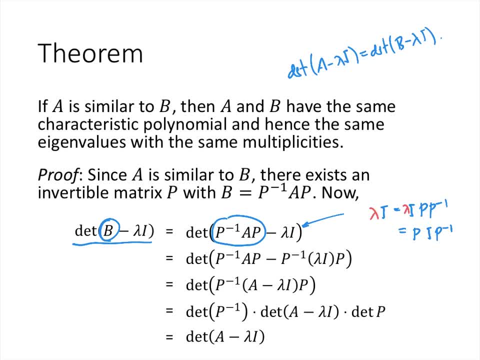 So if I multiply by lambda here again with scalar multiples in matrix multiplication, we can kind of put the scalar wherever we want, And the advantage of doing this is that now we have a P inverse on the left of both of these terms.